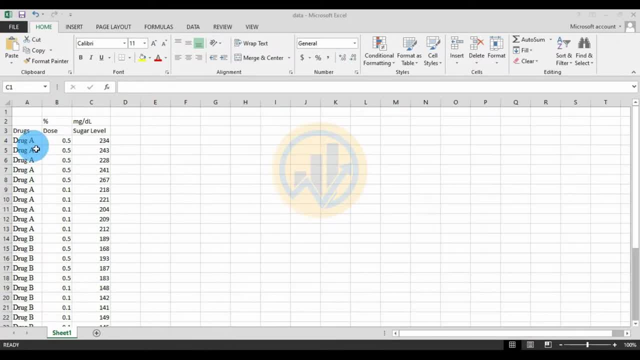 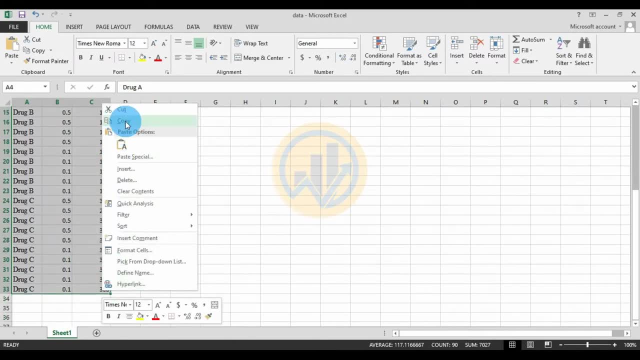 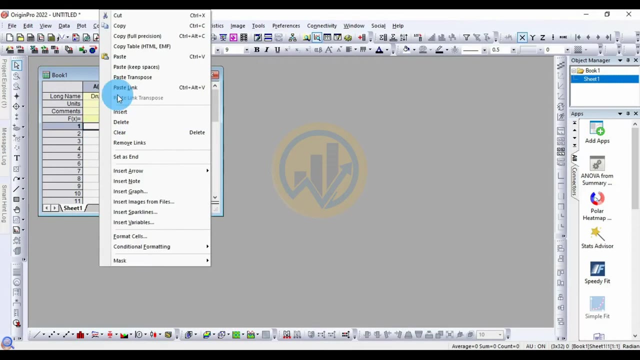 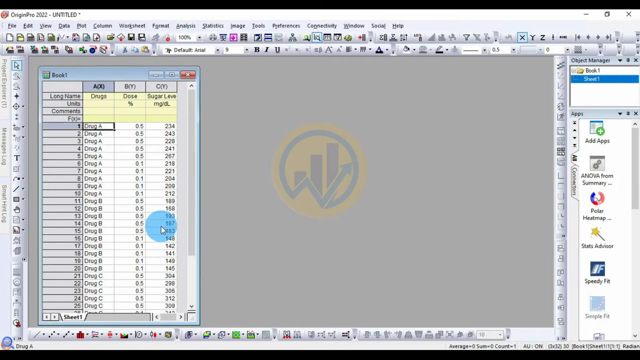 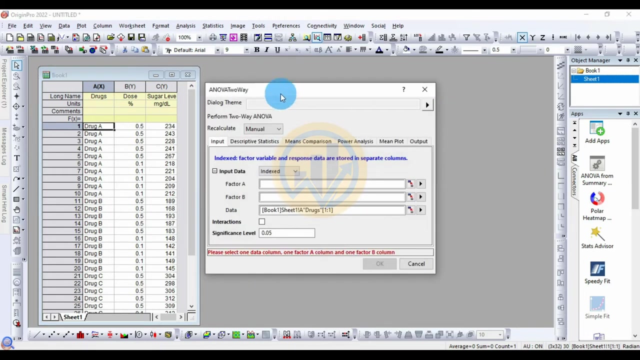 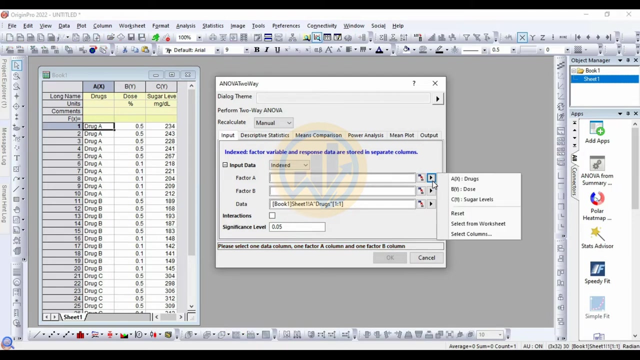 Okay, now copy the data. Copy, Paste the data. Okay, Then go to the statistics menu, the Hanawa, the sub-menu for the two Hanawa. open the new dialog, Then the input data for the factor A, the drugs three type. 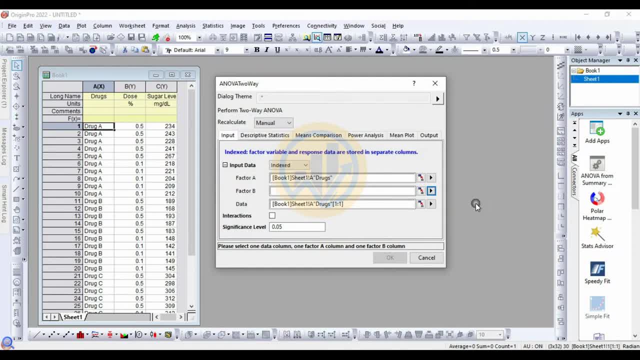 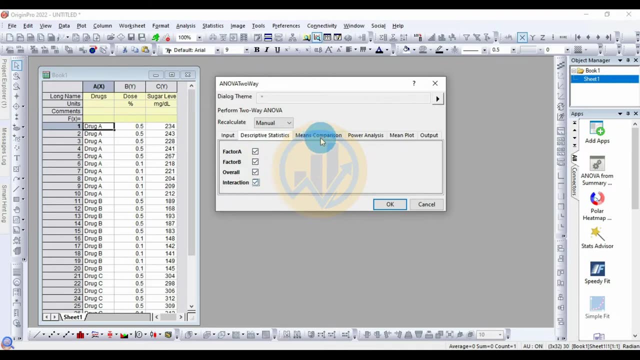 drugs under factor B for the dosage and the data for the sugar level. okay, then click the interaction button. then go to the descriptive statistics menu. they click the all the box, factory a- B, over on interactions. then click the mean comparison- the bone fairy, then one for the mean flat, the interactions, then 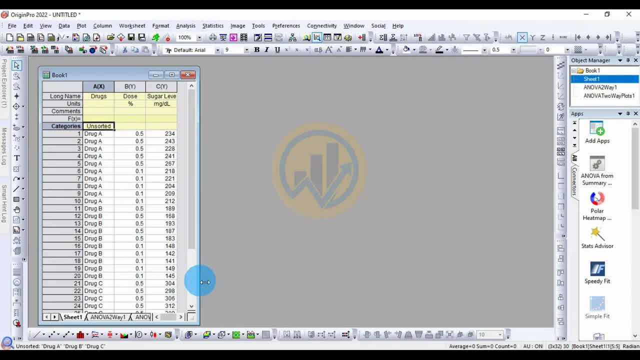 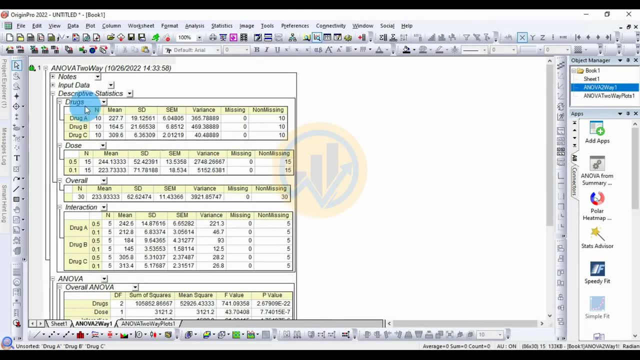 click the ok button, okay in the bottom layer, open. okay. this is here to an over the first one table for the descriptive statistics in the track table: the truck a, B, C and a total number of drugs, certain the 10, 10 and total number of trucks, the 30. the mean for drug a, 227 and the drug P. 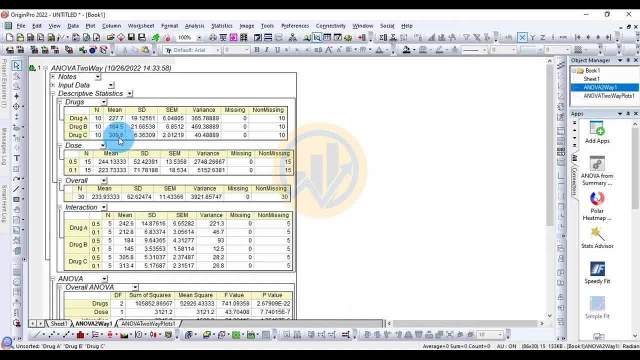 100, 18, 164. drug c: 309. and the standard deviation, standard error variation: missing data 0. the dosage. also missing data 0. the dosage type for the 0.5 percentage and 0.1 percentage. the overall for the data. the total number of sample: 30. the overall. the mean value: 233. 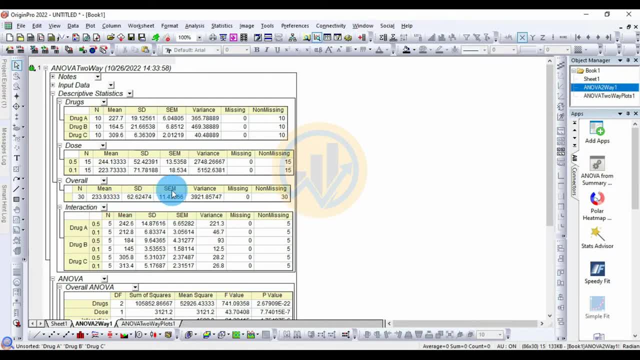 the standard deviation 62.62 and the standard error 11.43. and data also the missing data 0. then fourth one table for the interactions: the interaction for the drug a and the percentage, the dosage percentage track, a dosage percentage 0.5. the number of sample 5, the mean value standard. 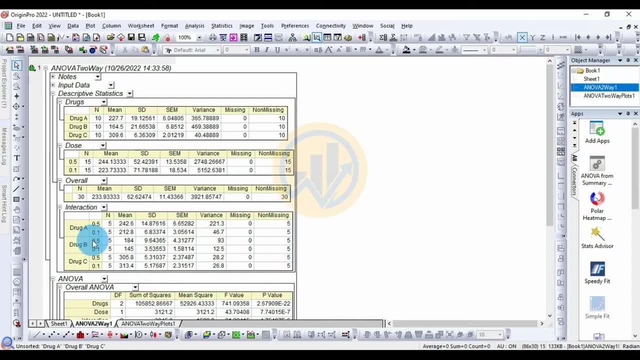 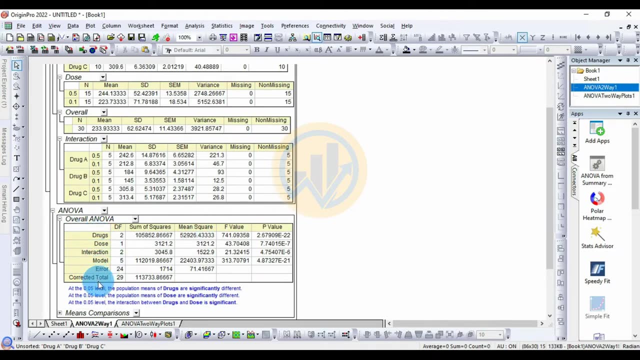 deviation, the missing data, also the zero. the drug p, the interaction for the dosage 0.5 and 0.1. the drug c: also interaction for the 0.5 and 0.1. the next one, the important table for the two on our table, the dosage, drug interactions, the model error and the total. that uh, truck, that uh. 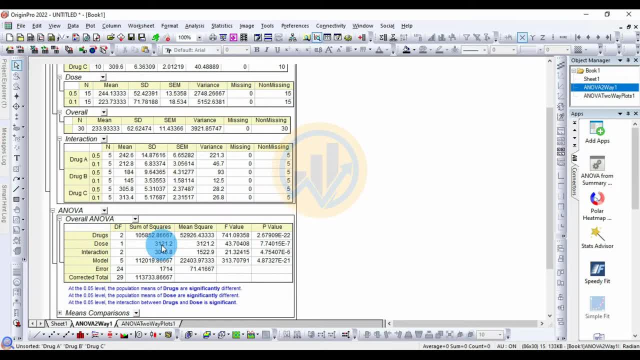 difference of freedom. the two, the sum of square, the one lakh fifty, uh, five thousand eight hundred and fifty two, the mean square, uh. fifty two thousand nine hundred and twenty six, the fle for four hundred forty one point zero nine. the p value, the scientific value, this value converted method for the. 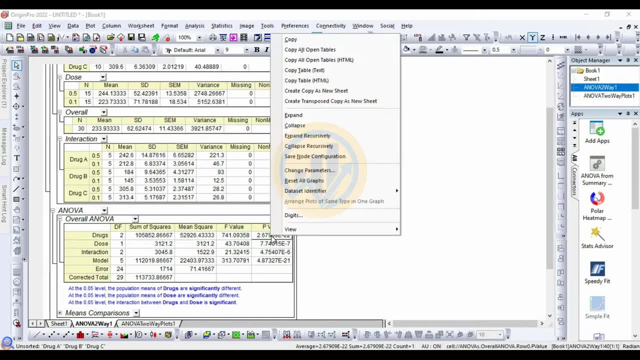 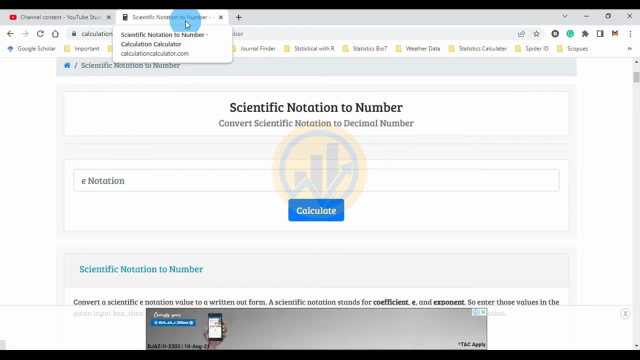 normal the numeric number, copy the value, go to the chrome, the already and open the scientific notation to the numeric calculation calculator- this link they mentioned. to the description box. they click the paste the data. they change capital e to small e. they click the calculate button. this is a significant value. 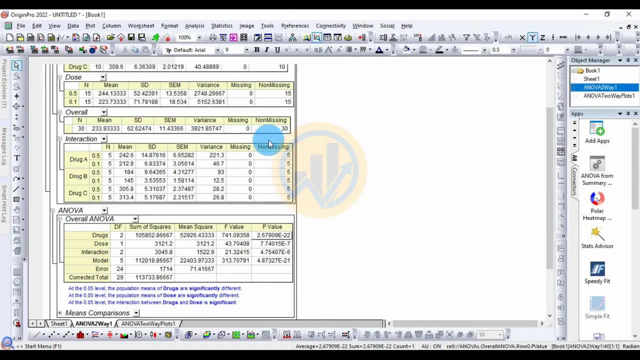 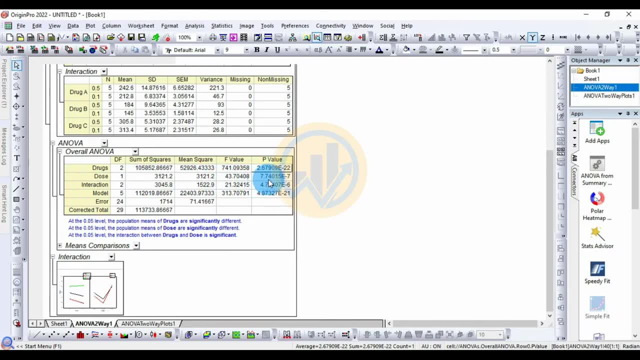 0.00, then go to the origin pro software. okay, then next on dosage, the dosing for the f value 43, the significant value 7.474 and the interactions under the model. then, at the 0.05 level, the population of mean drugs are statistically significant, the drug is also statistically. 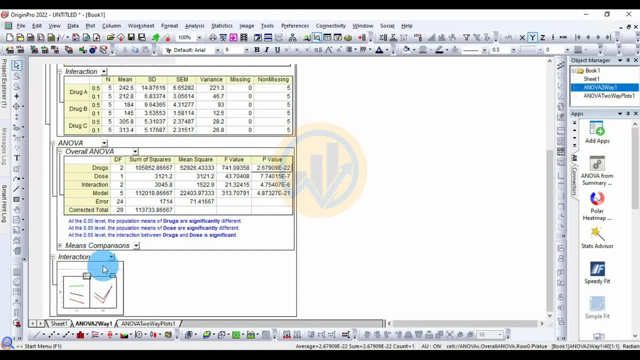 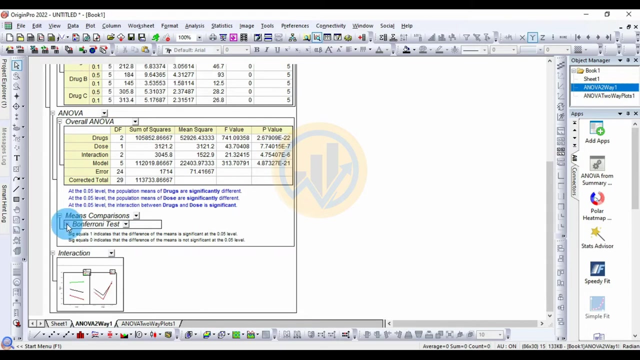 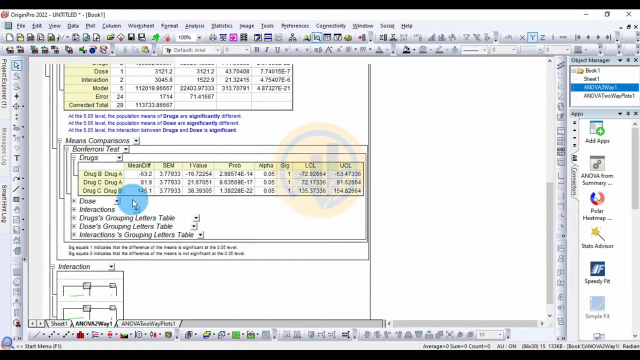 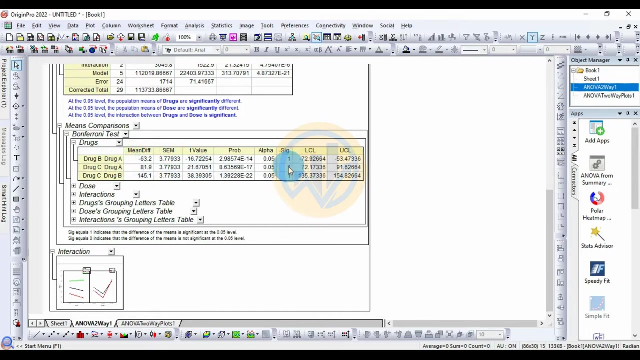 significant: 6., 9., 10., 11., 12., 13., 14. 15.. drugs: open the table the drug b and drug a. the comparison for the significant value one, the our standard significant value 0.05. the one indicator below the mention the next the. 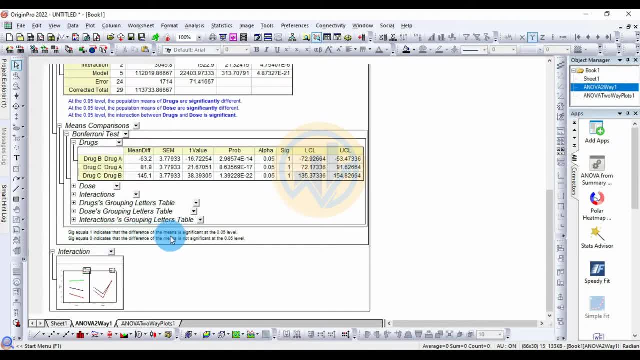 significant equals one indicator that the difference of the means the this significant at the 0.05 level. the zero indicated that indicated the means the not significant. there are also the truck e and the key as a statistically significant, drug c and the drug a, also the statistical significant, and drug c and drug b also the statistically significant. 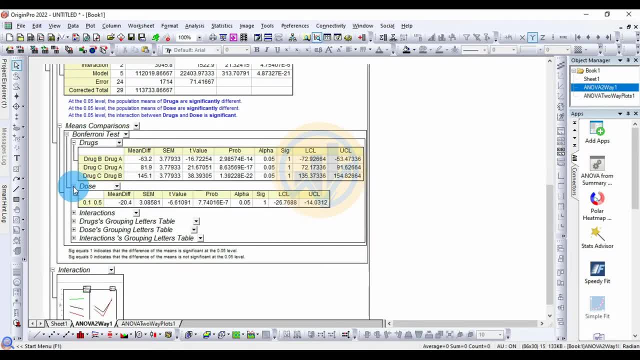 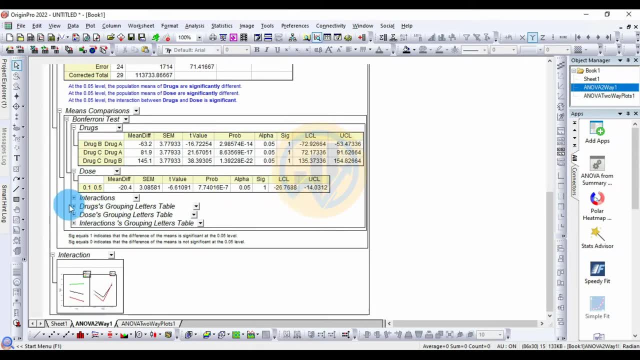 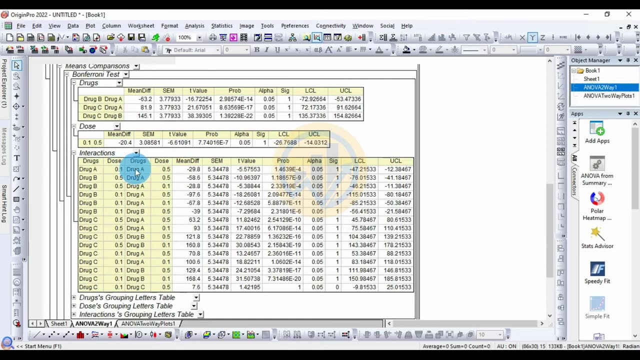 the next one for dose table: click the plus icon. the plus icon doses 0.1 to 0.5 %. that also the statistically significant. and next one table for the interaction table. okay, the drug. here the dose is 0.05 and drug here. 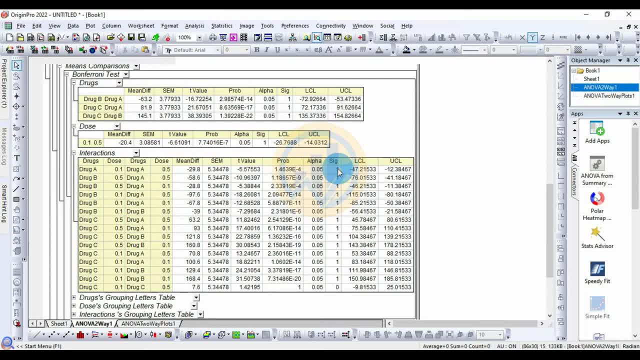 The dose is 0.05.. That also the statistically significant. Then next one for the drug B: 0.05.. Drug A: 0.05. comparison: The statistically significant, The non-significant. for the drug C: 0.1%. Drug C: 0.05%: That statistically non-significant. 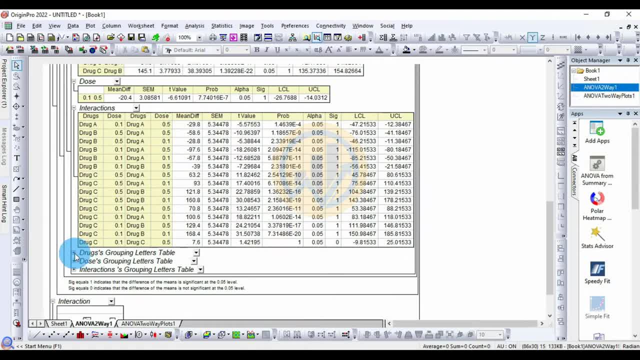 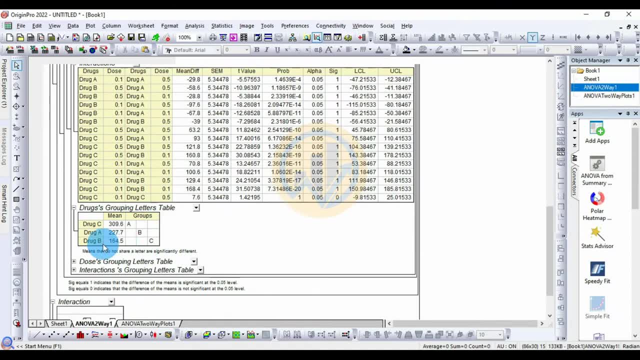 Then next one for the drugs group letter table, That one important, The result for the highest sugar level control for the best performance for the drug B. And the second one for performance for the sugar control level in the drug A, The very poor lowest drug for the drug C. 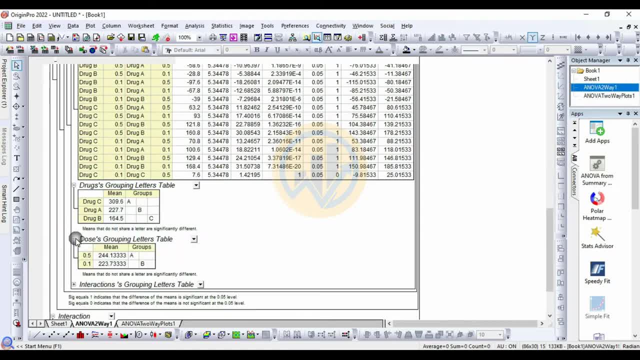 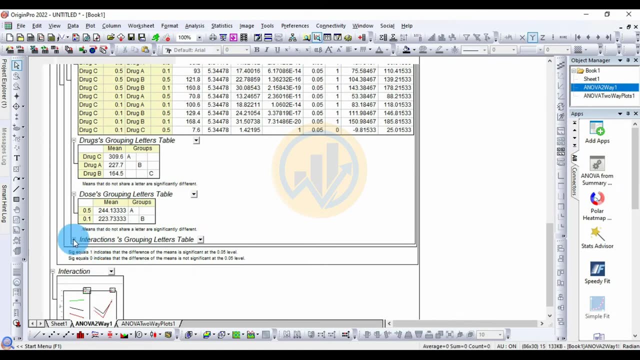 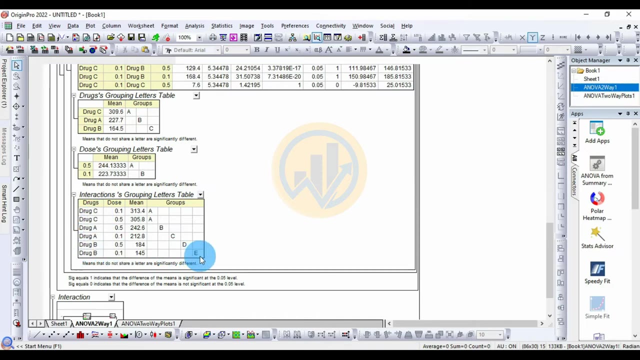 And the dosage group letter. That also the dosage. Click the plus. The dosage 0.1% is the best, sugar control And 0.5% is the second on the sugar control. Then interacts group in the letter: Okay, Then drug C, the drug B, and 0.1% is the best, the sugar controlling method. The drug B, also the C, that is stable. 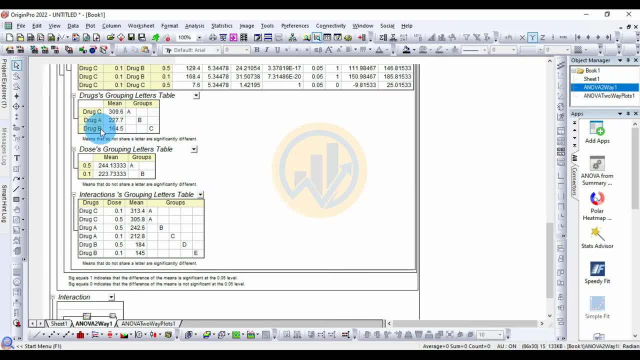 Drug C is. drug B is the best sugar control method, But drug B is 2. Certain types, the concentration 0.5% and 0.1%. That also the important part for drug P. 0.1% is here Best sugar control in blood. 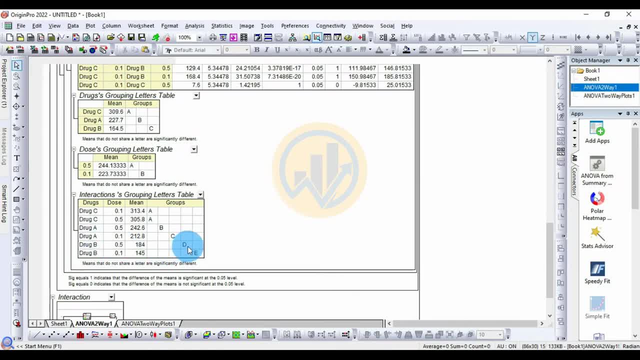 The next one for the drug P. the 0.5% % is next to the sugar control, The best for the 0.1% and 0.5%, The 1st for the 0.1%, 0.1% and the fourth one drug A: 0.5%. the drug C: 0.1 and 0.5%. also the very poor performance. 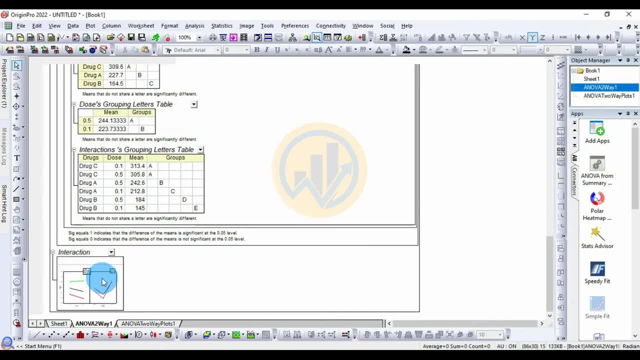 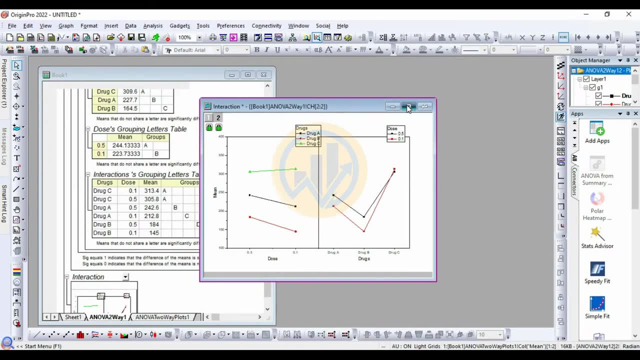 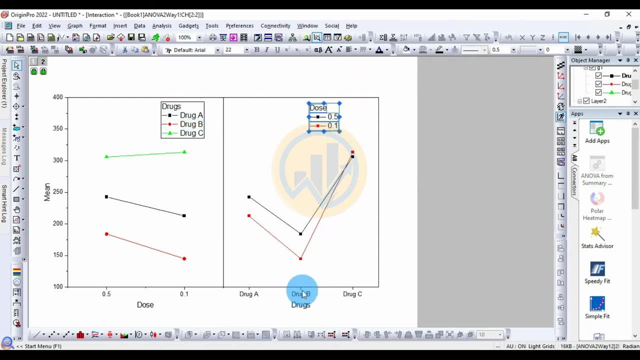 for the blood control, the blood sugar level. okay, next one for the platinia two-way ANOVA. double click the plat. open the new window. this plot also explained for the table the drug P for the best performance for the 0.1% sugar control level and 0.5% is next on the sugar breast control level. click the double. 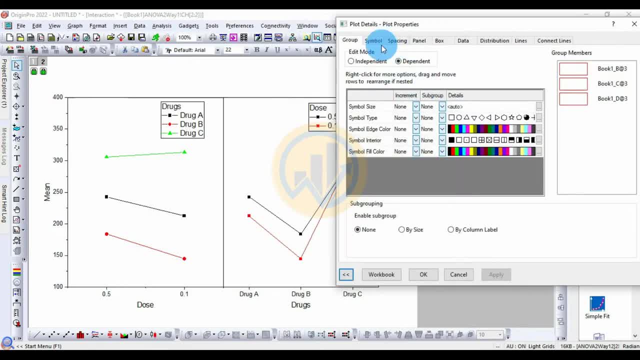 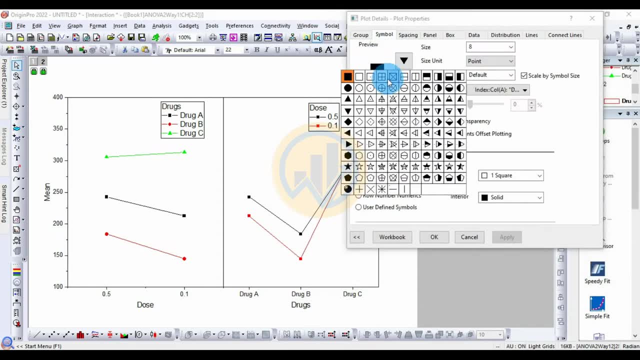 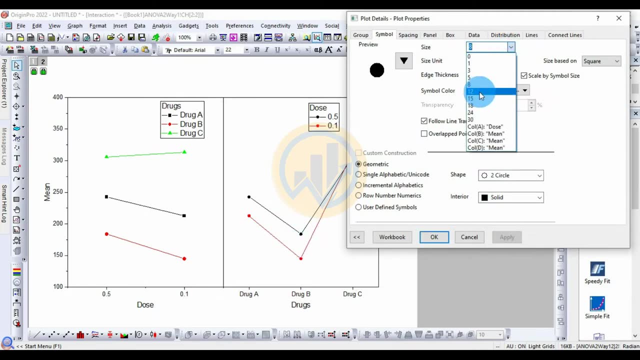 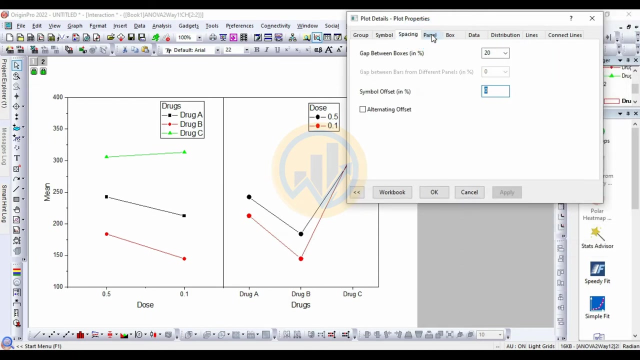 click for the line. open the new window. simple, you like? change the simple: any simple size. ok. change the simple: increase the simple size: okay. under spacing banner box: the data, the line, the connected line. change the symbol: increase the symbol size: okay. under spacing banner box: the data: the line, the connected line. 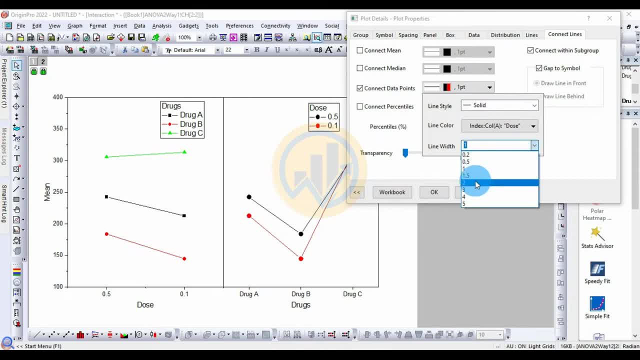 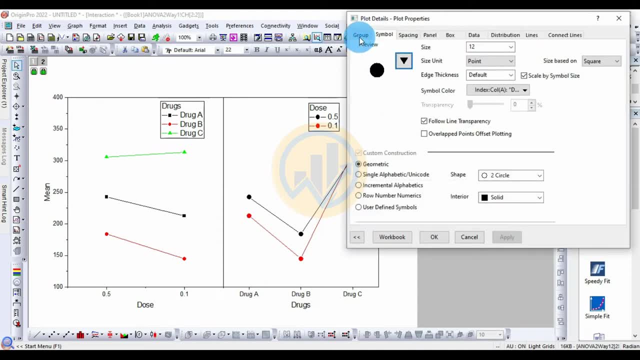 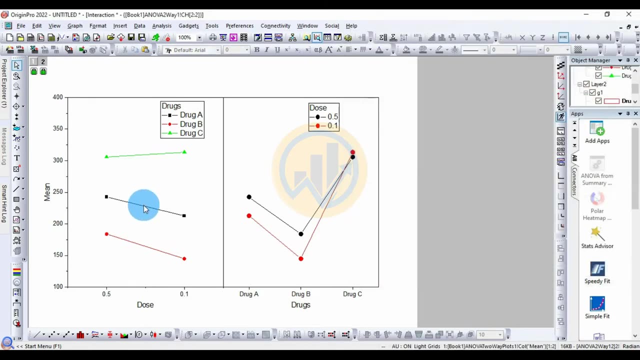 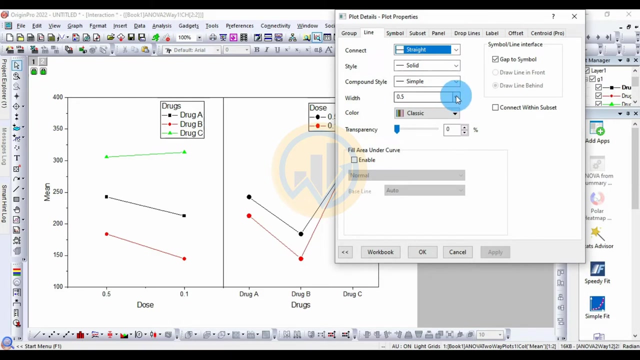 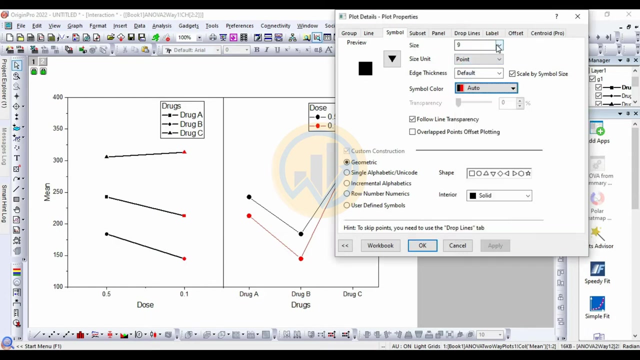 English for the line with it to simple: okay, the click for the trucks, the line icon, go to the line. we think it is about the two. okay, I think is three. then change color for the change color. okay symbol. also change 12 arrow. then apply a simple color: black and red, auto or point by flat. okay, then. 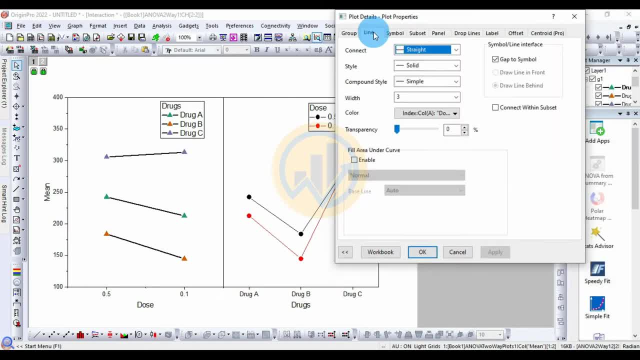 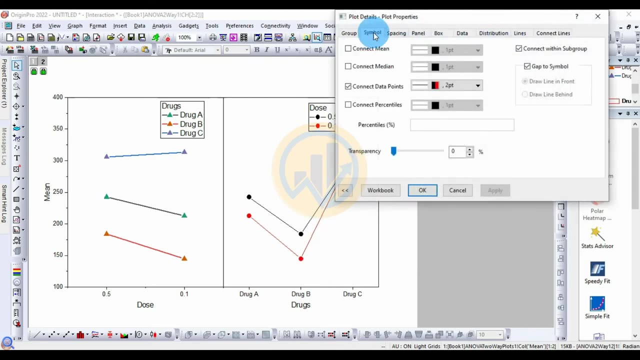 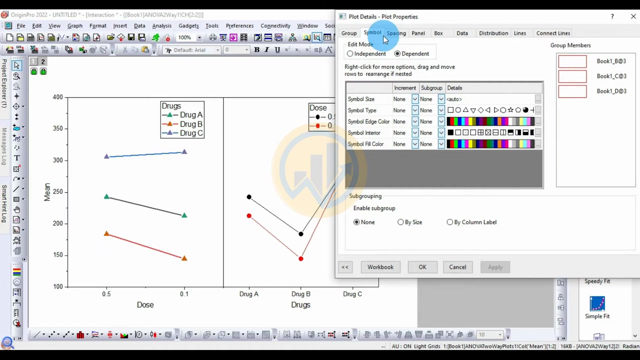 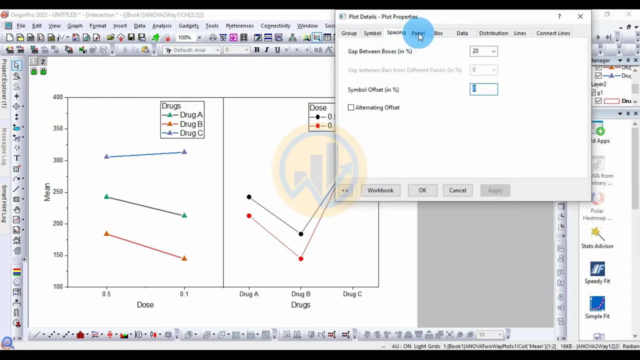 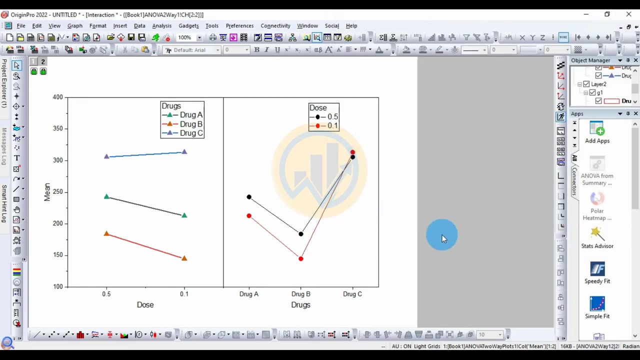 group line. also change color. then double click this, the with it. simple group line: simple, you, you, you, you, you. okay, then under the next one part of the truck- yet Battlesay truck is exactly the truck, the plot. under another one for the pouty. then the extra part. 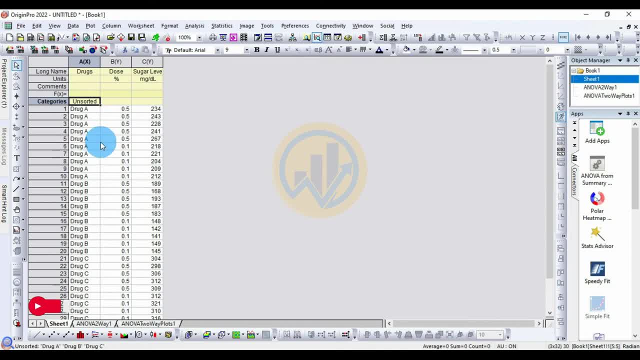 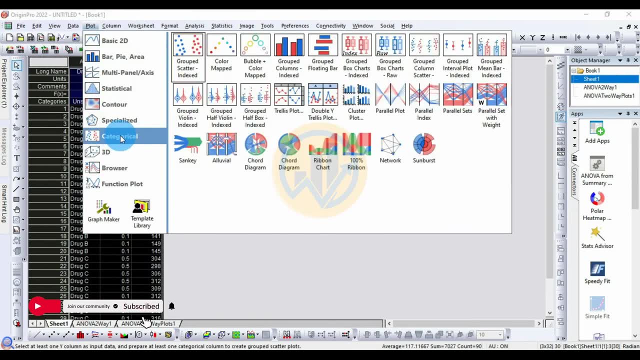 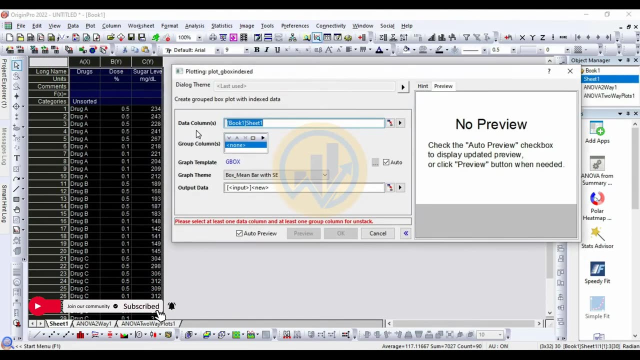 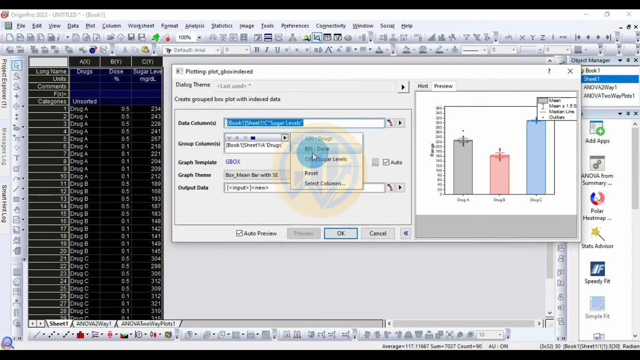 this data: how to земce a PDX 2.0. set up the whole the data cot, the flat me know and the court. the category can under clip the group mean bar, open the new window. first cell for the data column. so go level. next add the group level the truck under the dose. okay, the group things for the 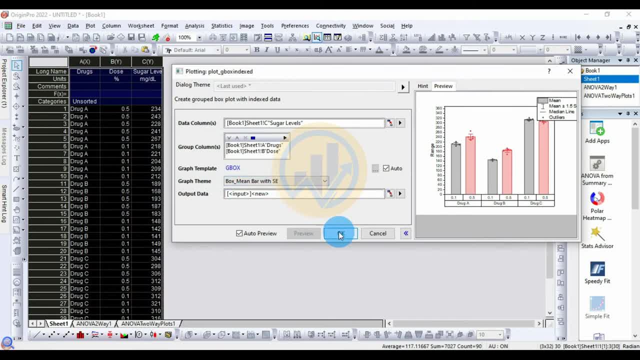 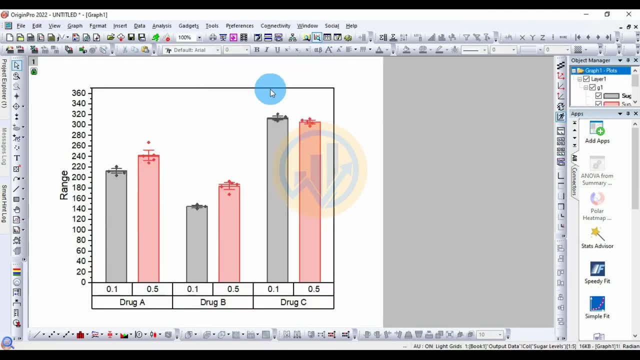 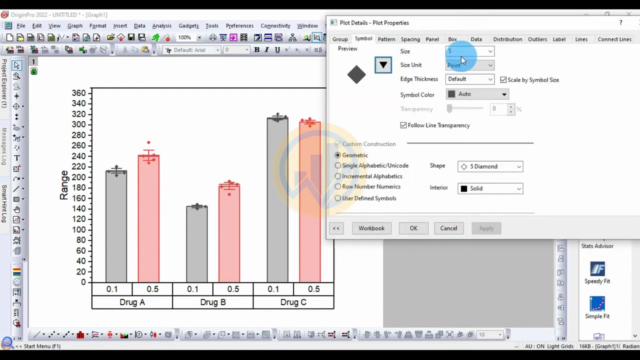 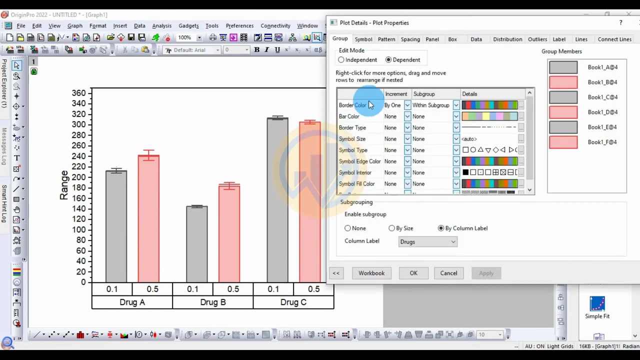 box box plot bar. with the standard error. then click the OK button with this okay, double it for the graph. open the new window. the change for the simple: 0. then reduce for the simple: under the group color: the border color. under the bar color: change the bar color one by one under within the group click: change the. 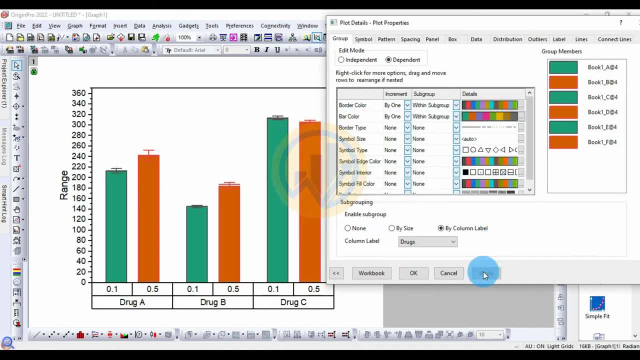 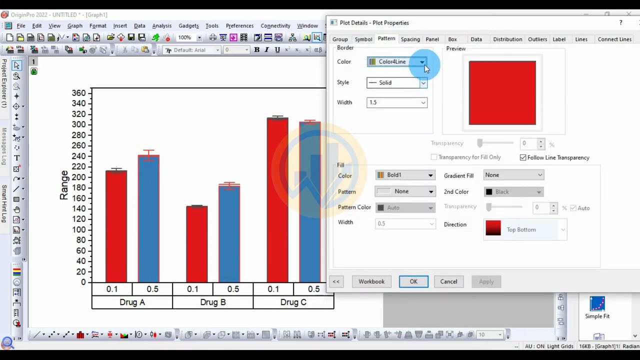 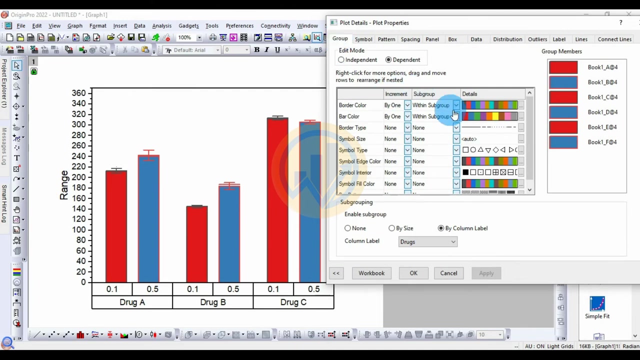 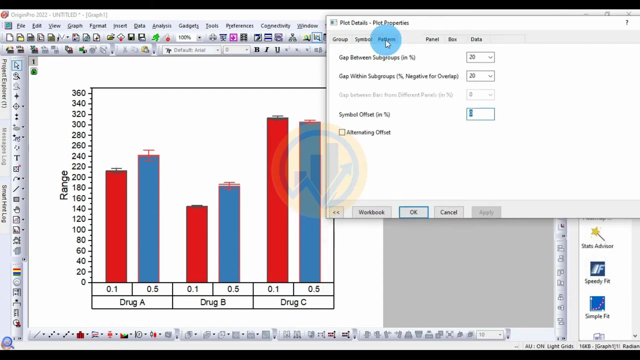 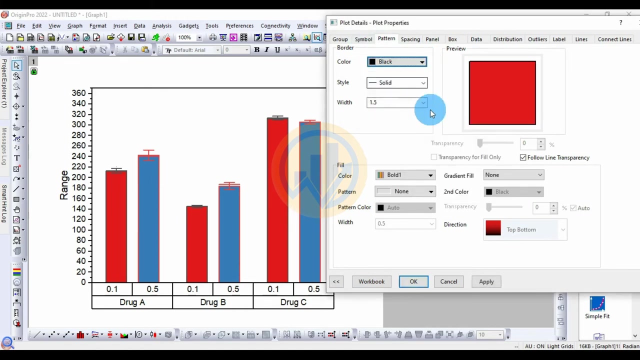 bar color. okay, change the color. if you like any color, change it blue color line for okay. okay, then one border type and go to the simple, the pattern. next one, the border color box. then I'm spacing: single color. okay, then click ok, single color. the width increase to 2, then apply 3. okay, then change the. 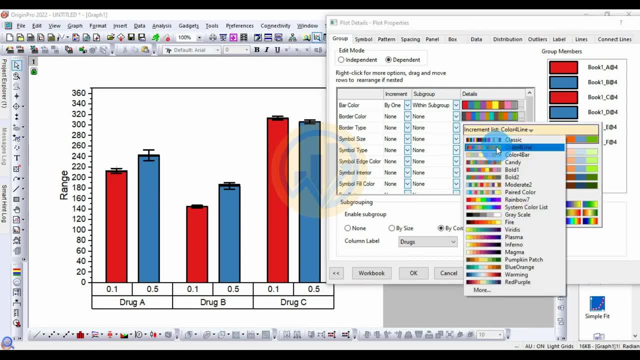 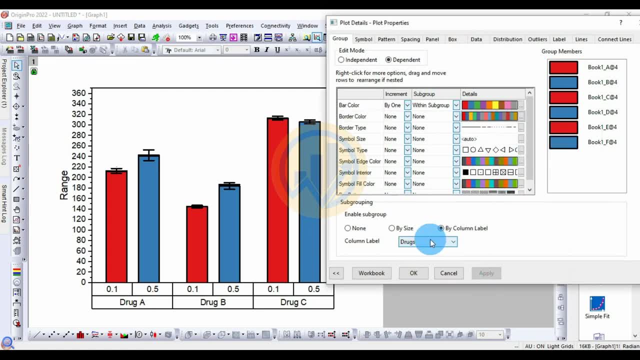 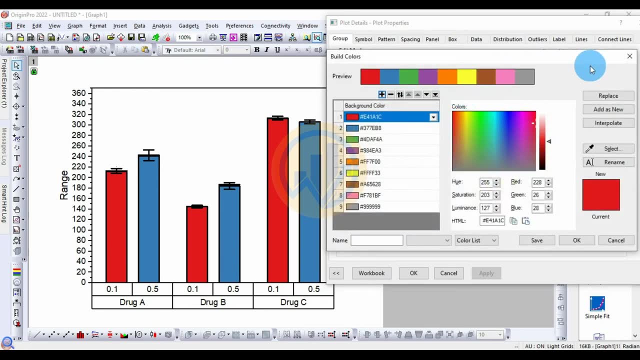 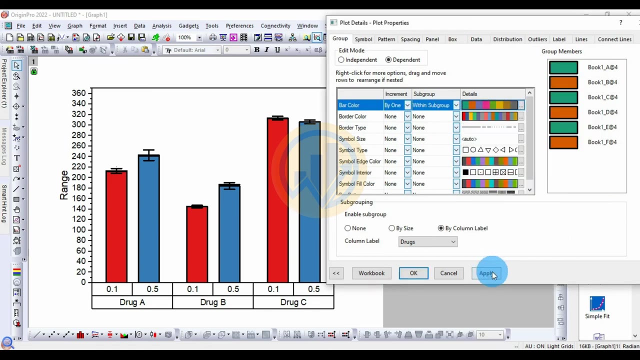 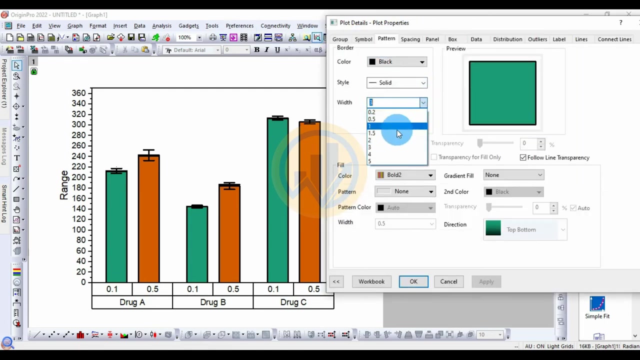 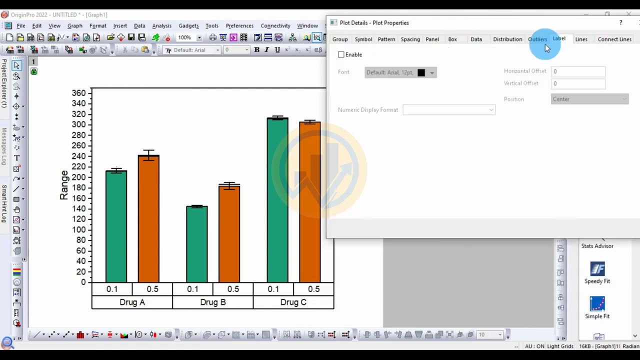 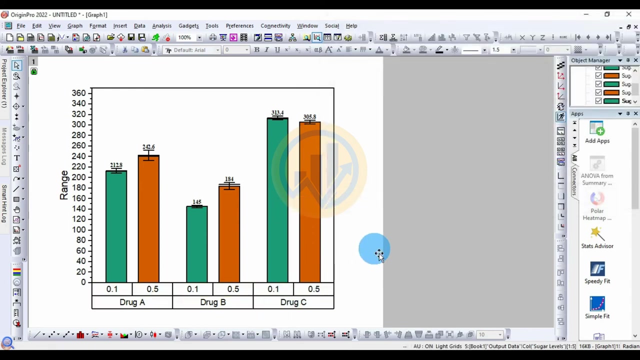 different effective color: classic 4 and candy. okay then then I'm spacing the pattern, the reduce size for that to okay. then then for the label, click the enable button, change the font for the time Roman. then click the plane. they click the board outside the hint. yeah, then click. OK, then double click for the X bar.